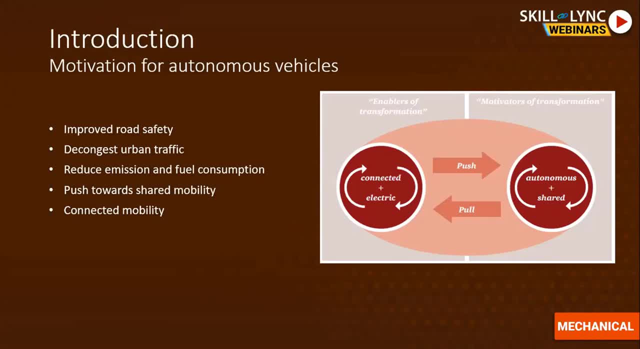 to communicate with the environment or the surrounding, for instance, automotive IoT. Now, in order to better understand the various levels of development in automation or autonomous vehicle development, researchers and developers have actually come together as authorities, like society of automotive engineers. they have come about with a serious 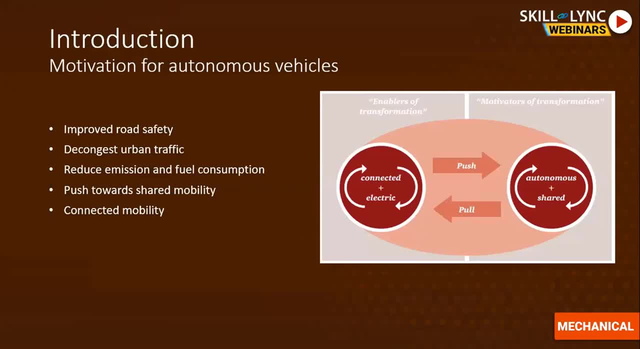 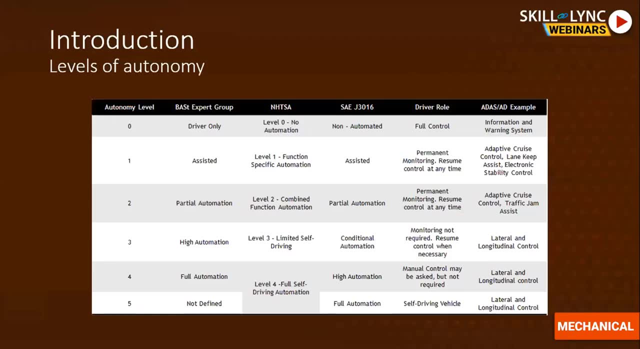 classification of autonomy based on the level of automation. they are classified into six levels, starting from level zero and going up to level five. where in level zero is no automation. where in the full control of the vehicle is with the driver. the ultimate aim of autonomous vehicles are to remove the driver from 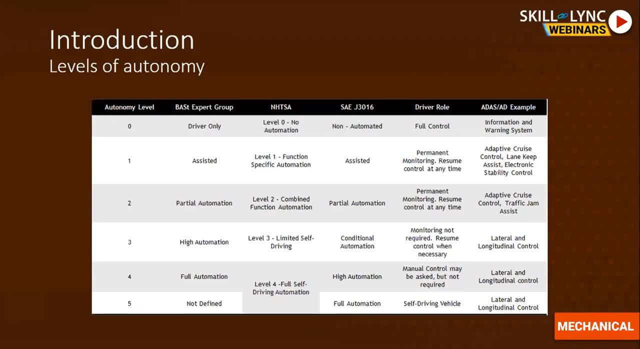 the vehicle control loop. the vehicle in itself is able to make control decisions, to navigate, to maneuver, everything is controlled by the vehicle itself. that's the ultimate goal. so, and each step towards that is classified into autonomy levels wherein we start with zero and which in which driver is in full control. 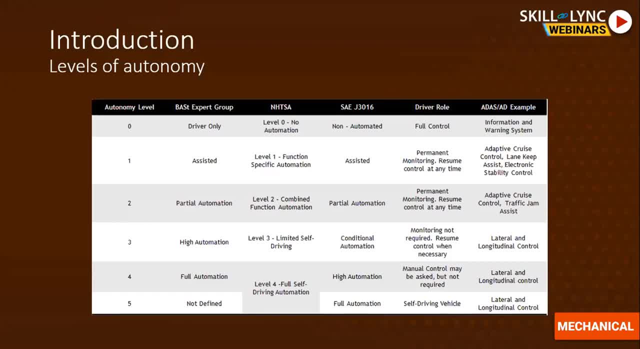 of the vehicle and you have certain advanced features like information and warning systems, like the parking parking sensors that we have in. you have certain advanced features like information and warning systems, like the parking parking sensors that we have in most of the cars nowadays as default and most of the cars that are available. 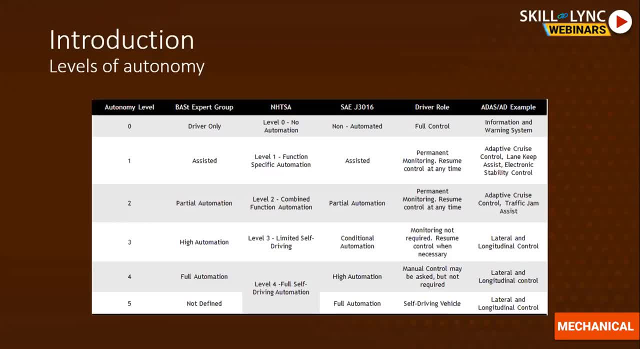 in India market are of level zero- autonomy, and then the next level is level one autonomy, which is like an assisted level. again, here also the driver is part of the vehicle control system and you have more advanced, advanced features like adaptive cruise control, lane keep assist, electronic stability control. 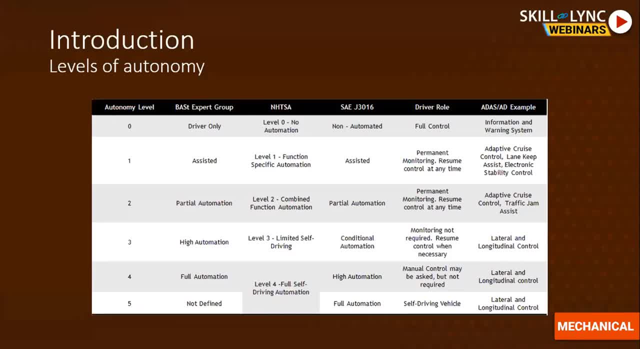 and it also include the features that were there in the previous autonomy level and it also include the features that were there in the previous autonomy level. moving forward to also, it's kind of similar. you have more additional advanced features, but again the driver is crucial or important part of the vehicle control. 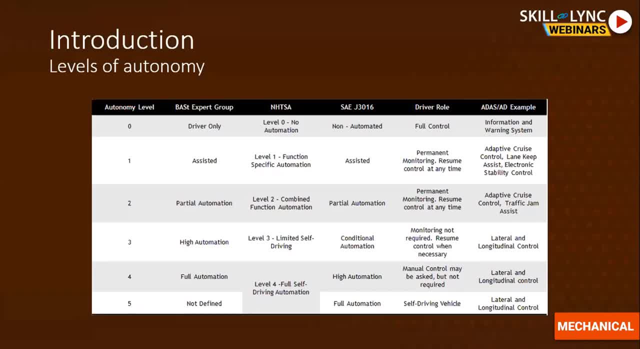 system. then we moved to level three. here is where the actual transformation happens, so wherein there is a transfer of control from the driver to the vehicle, here the vehicle will be able to make control decision and maneuver the vehicle on various infrastructure structure that is available, but then at certain critical scenarios wherein the vehicle is not. 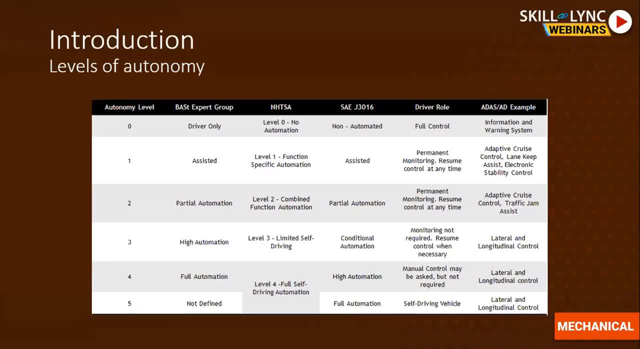 capable to make the control decision, the trans, the control is transferred back to the driver and the driver is made it has to be alert and to take up the control at any moment when the control transfer happens. and at this stage of autonomy level, the vehicle has the ability to. 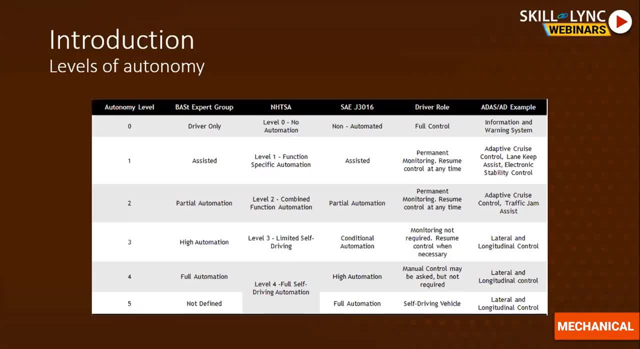 take lateral and longitudinal control. I hope everyone is aware with what I mean by lateral and longitudinal control. it is the vehicle's ability to steer and move forward and backward based on the requirements of the motion. then you have level four, in which it is high automation or full automation. some call and then again here the vehicle, the driver, is totally out of. 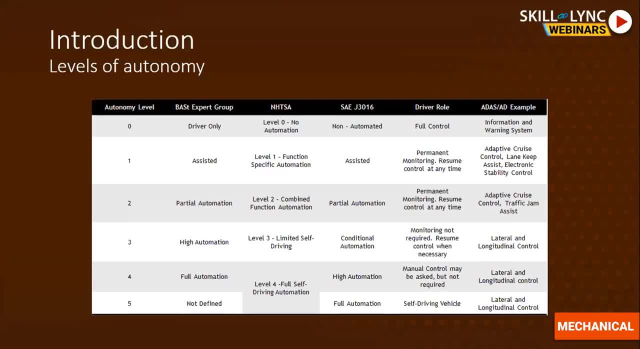 can be totally out of the vehicle control loop. then you have the level five, which is full automation, and then again here, the driver is totally out of the vehicle control loop and we have a self-driving vehicle. so there are a lot of projects that is going ongoing on level three and above. let's move to the next slide. so here, 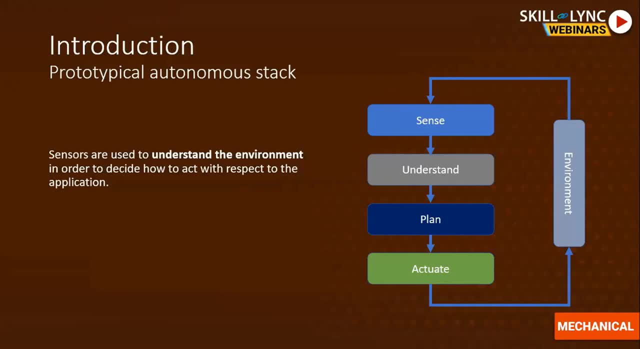 we'll be seeing the basic prototypical autonomous stack or the basic setup of an autonomous system. so the ultimate goal of the autonomous system is to replace the driver. how the way? how to achieve this is by giving the vehicle the ability to sense its environment and making it understand what the 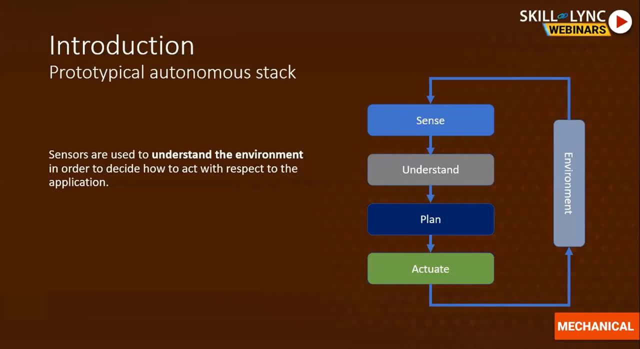 environment, how the environment is, and planning the motion accordingly and giving actuation signals to these systems accordingly. so here we have, we see, and so this entire component, the sense, understand, plan, actuate, this entire stack comes inside the vehicle and the environment is outside the vehicle. and this is again a basic generic autonomous system architecture. 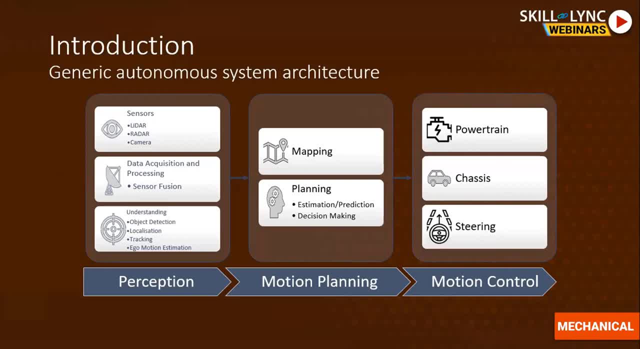 or this is not a detailed version. if you go to the autonomous systems development, any researcher, they would go for a more detailed architecture, where in they will be having more components, but this is the basic architecture in order for you to understand. so here we have the. basically, the system is classified into. 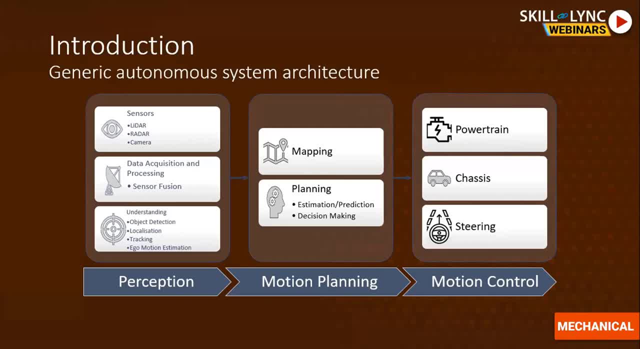 three. one is the perception system. then you have the motion planning system and the motion control system. the perception system takes into management system, takes into management system and the perception system takes into management the perception system and the perception system takes into management the perception system. and the perception system takes into management. 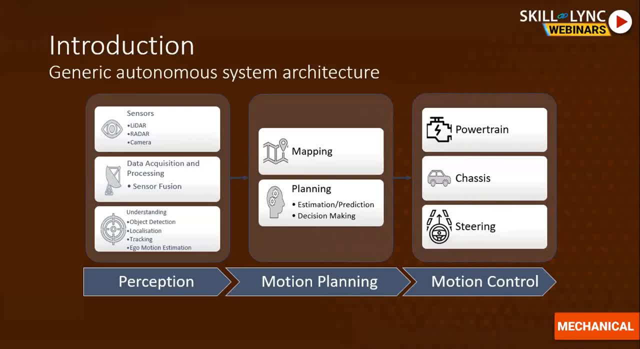 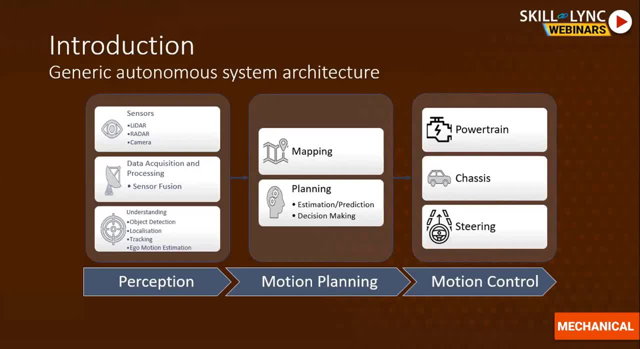 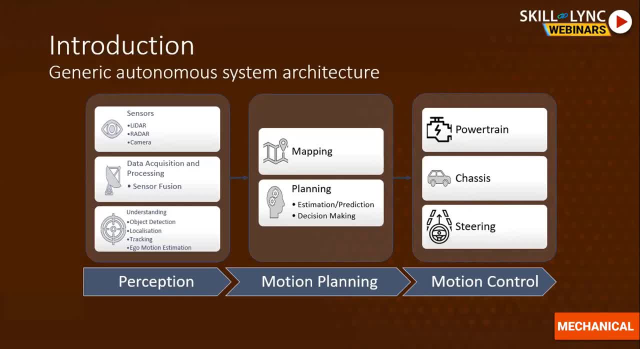 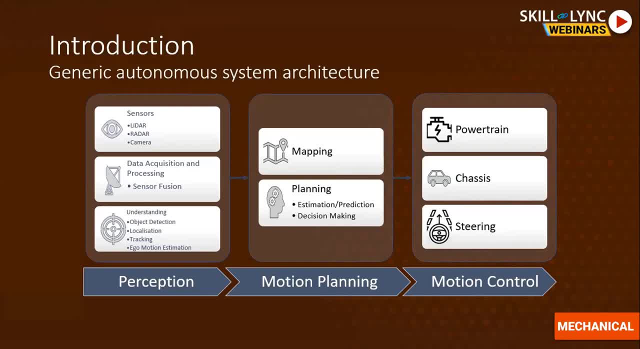 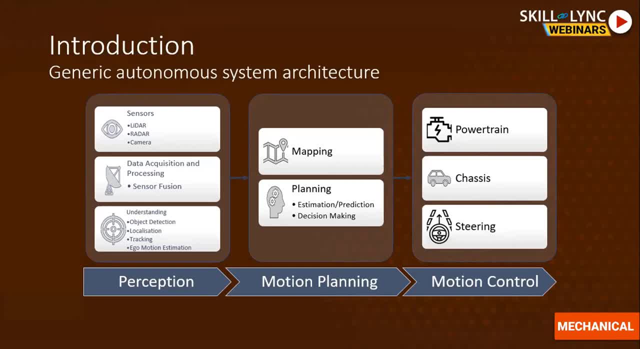 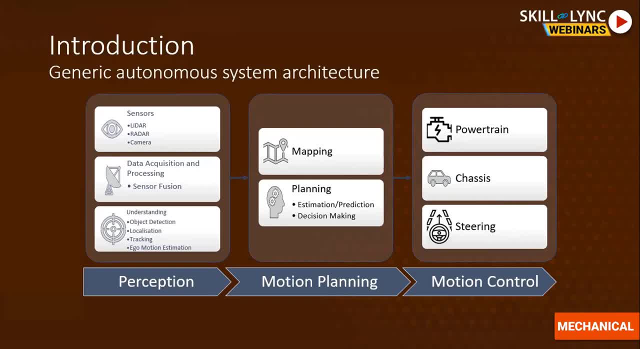 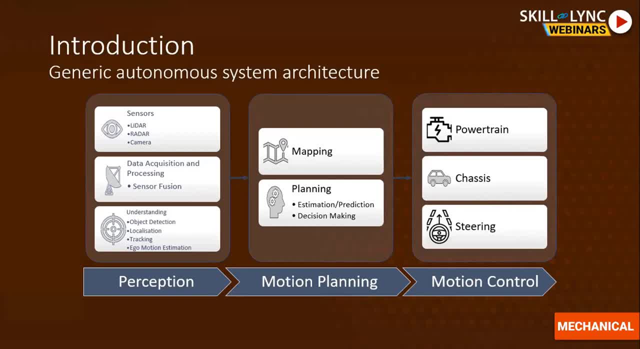 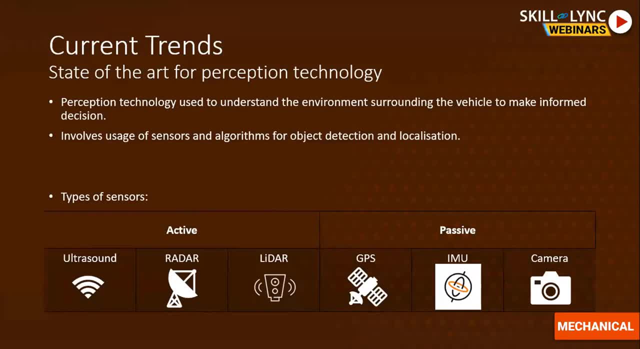 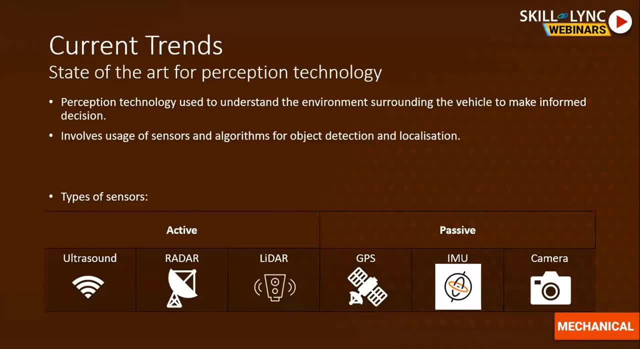 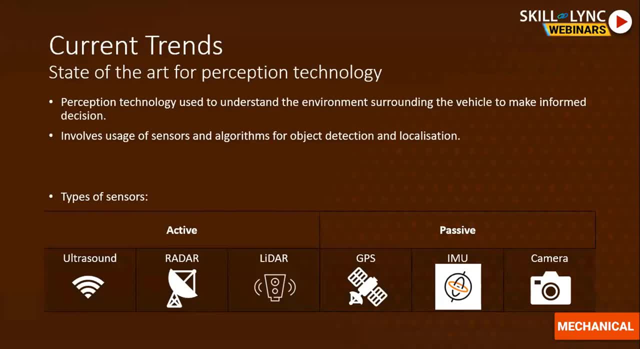 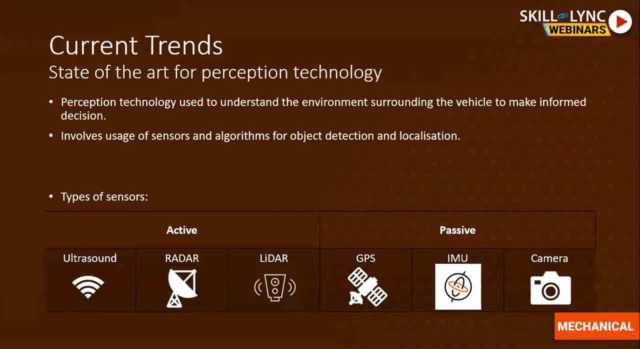 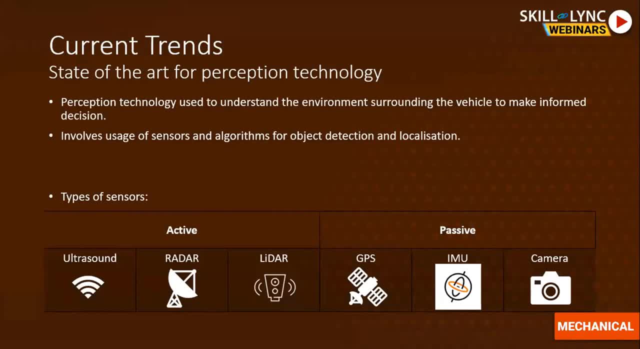 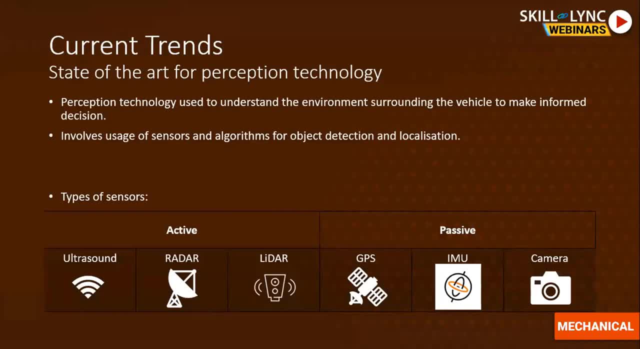 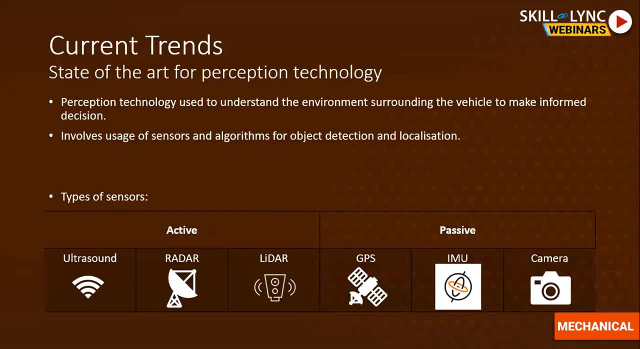 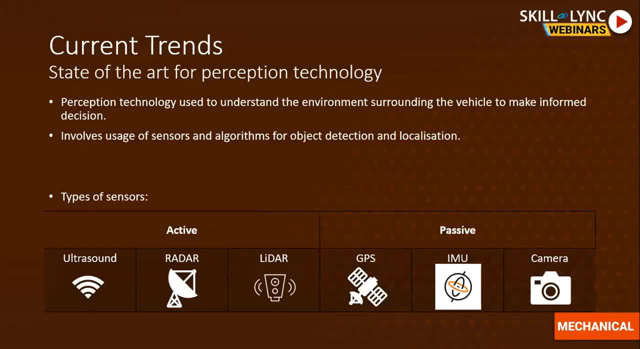 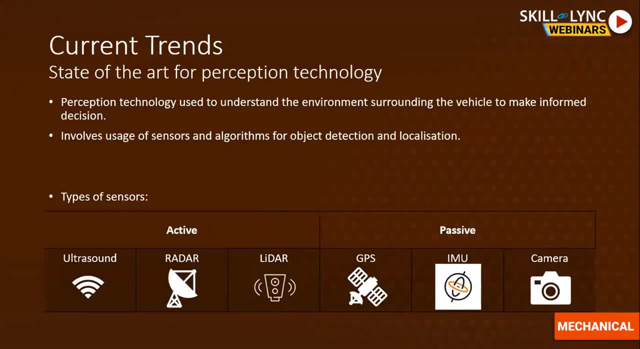 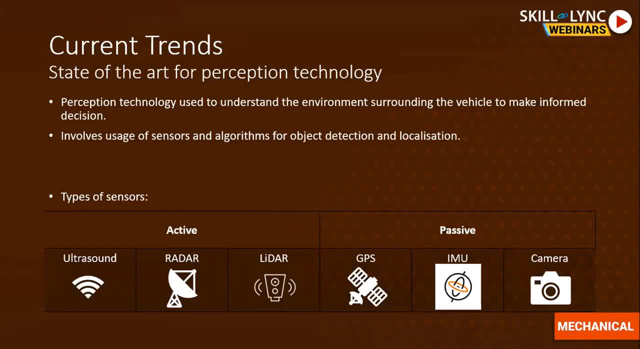 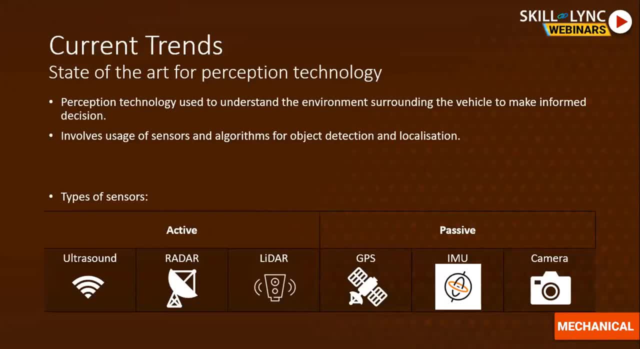 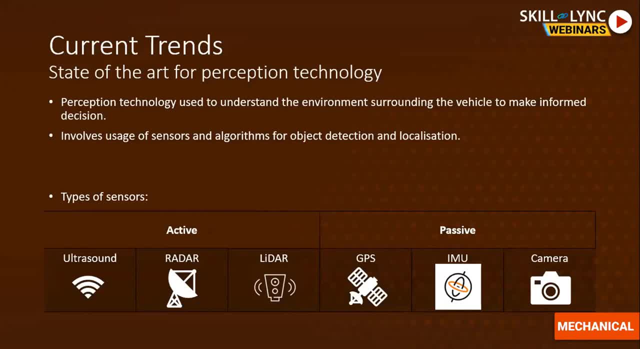 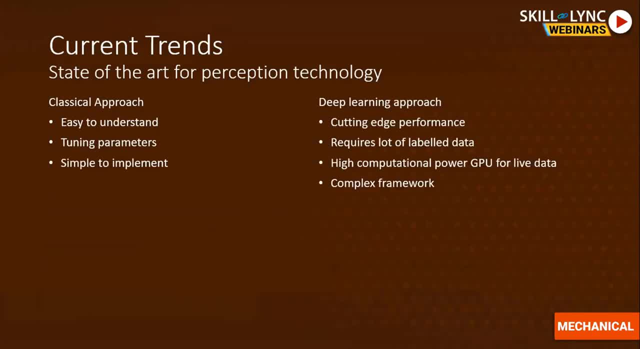 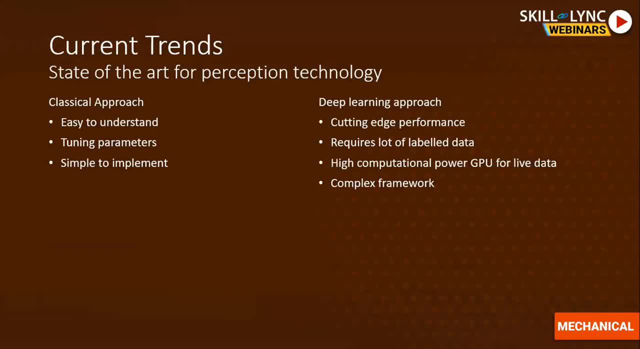 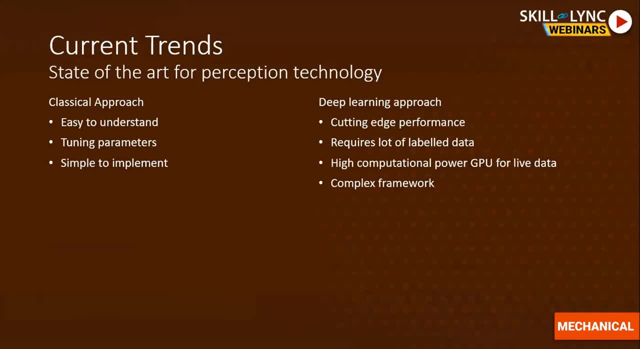 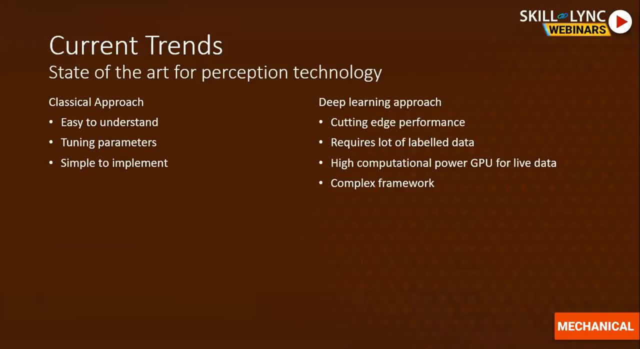 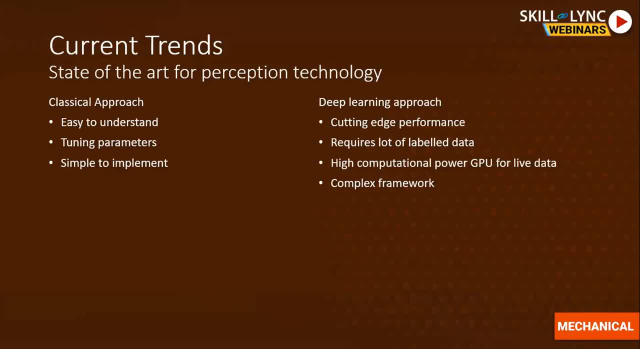 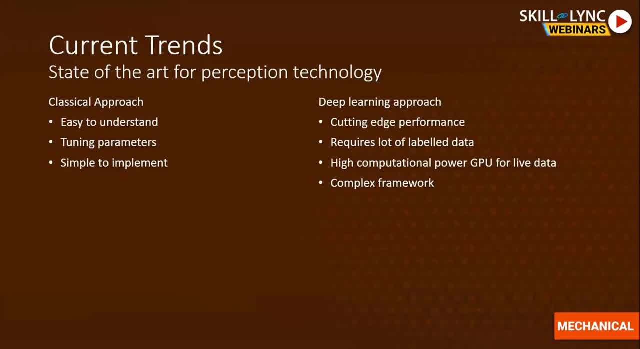 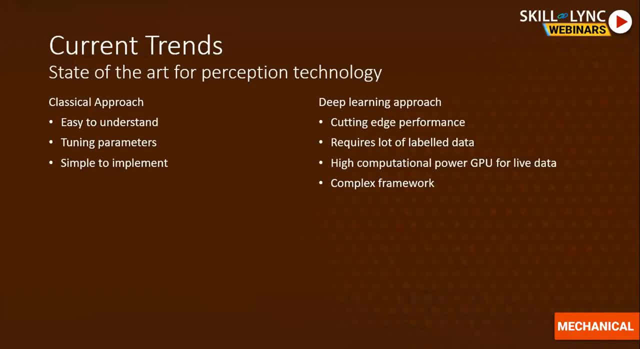 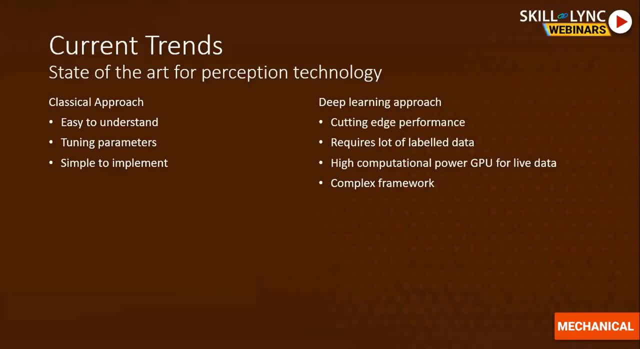 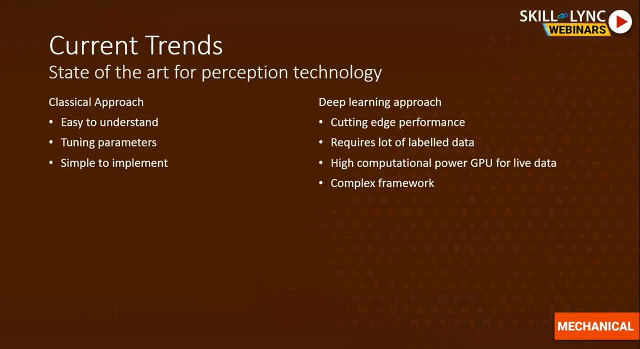 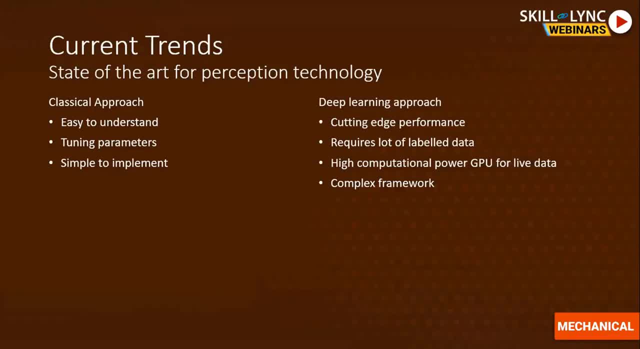 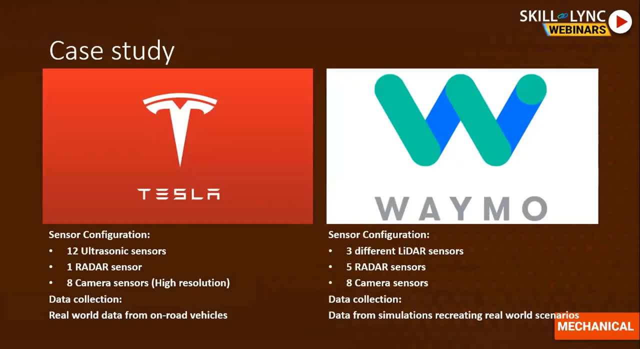 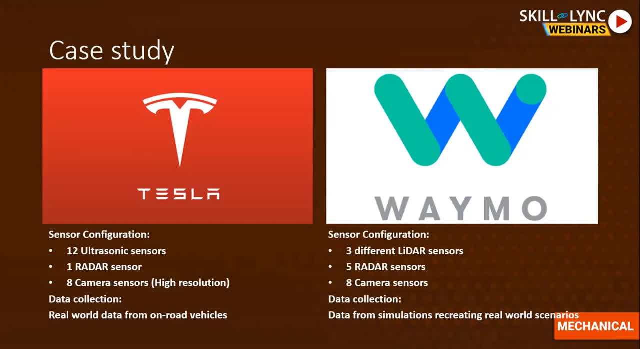 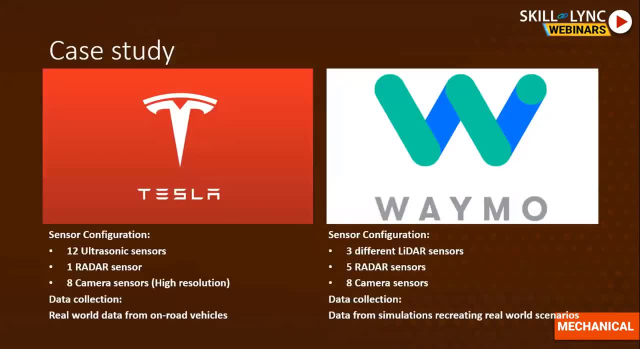 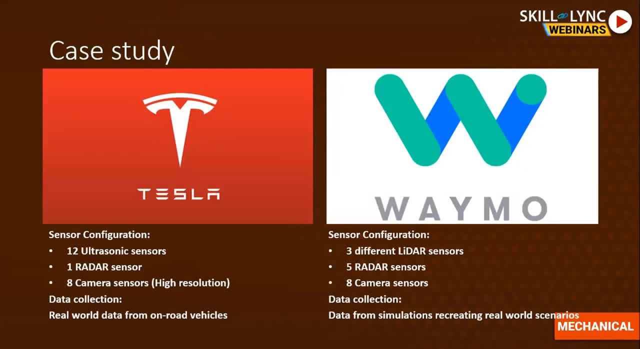 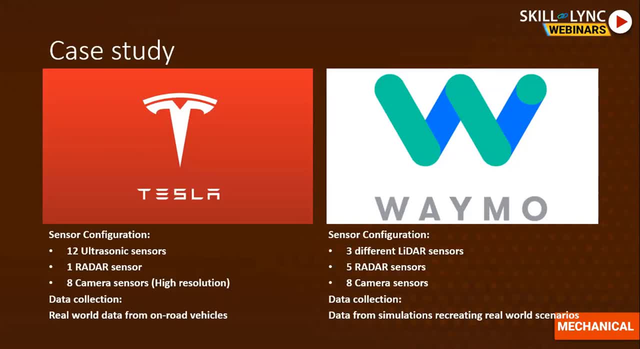 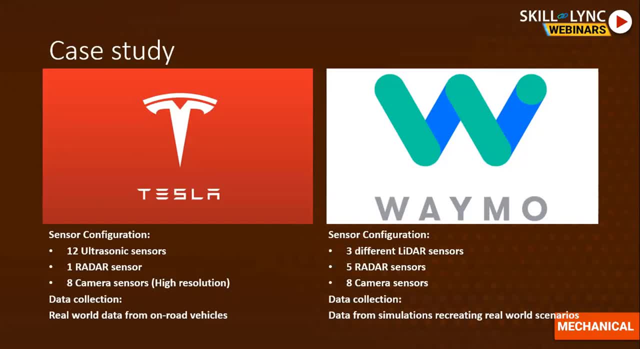 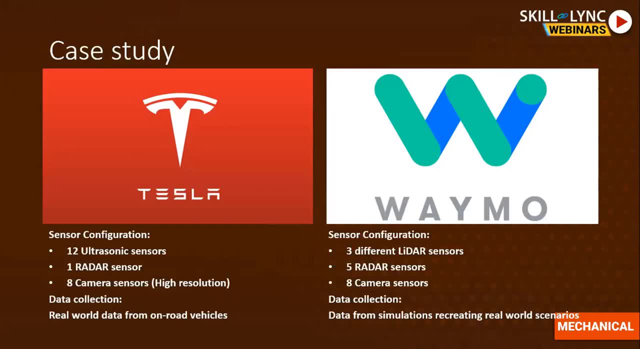 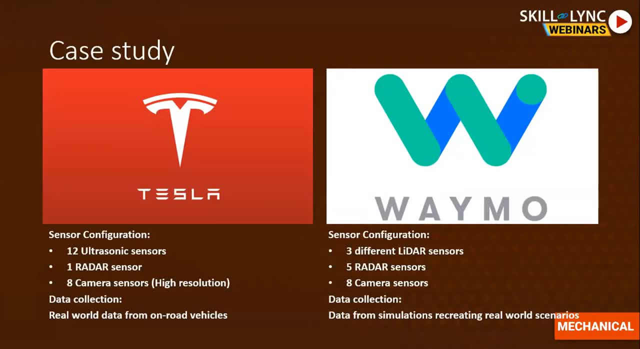 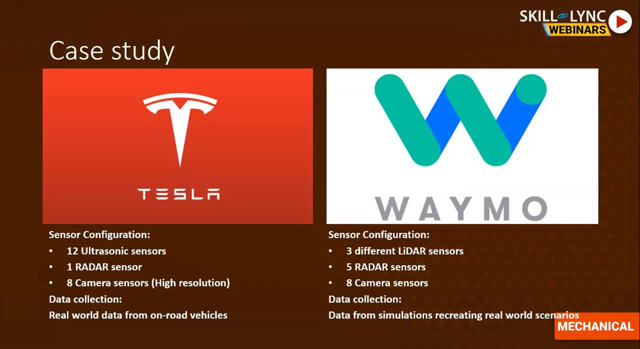 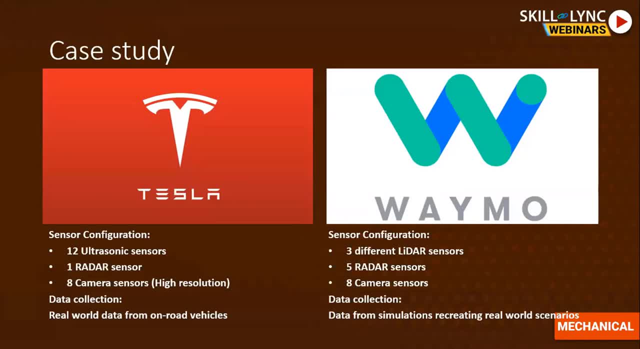 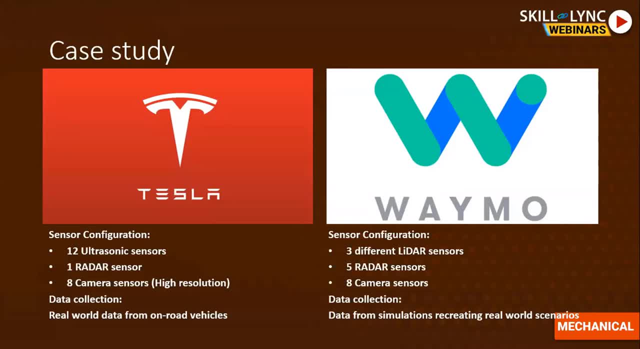 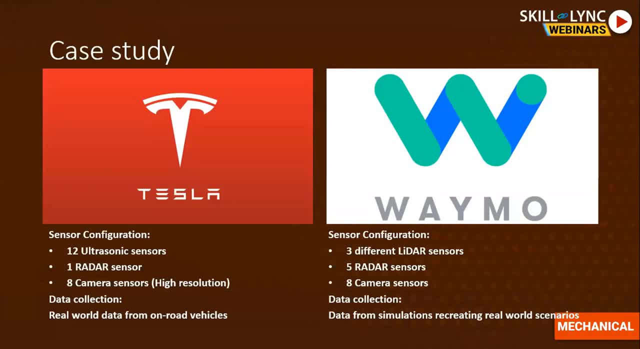 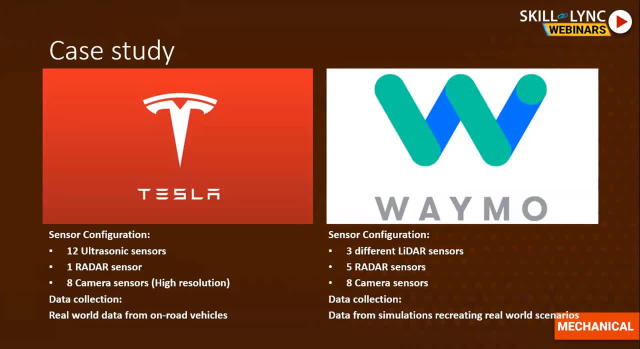 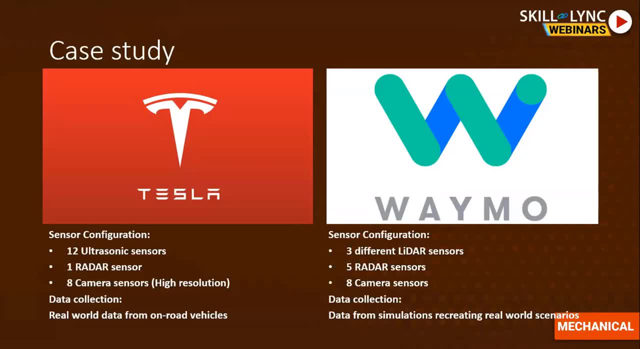 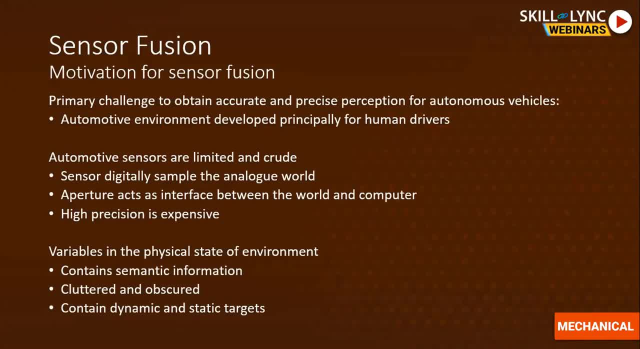 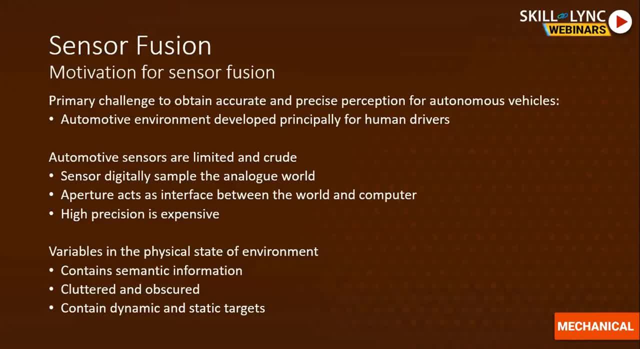 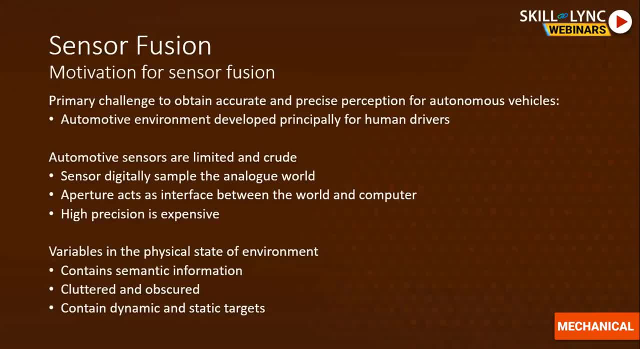 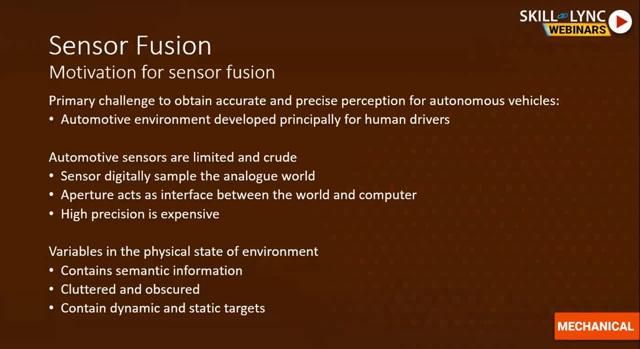 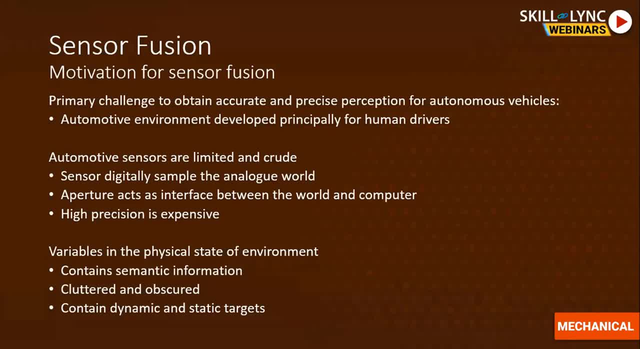 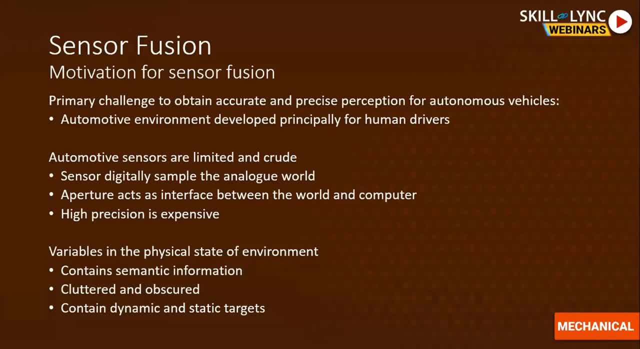 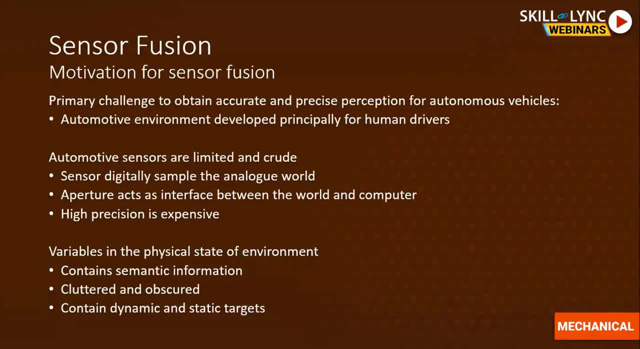 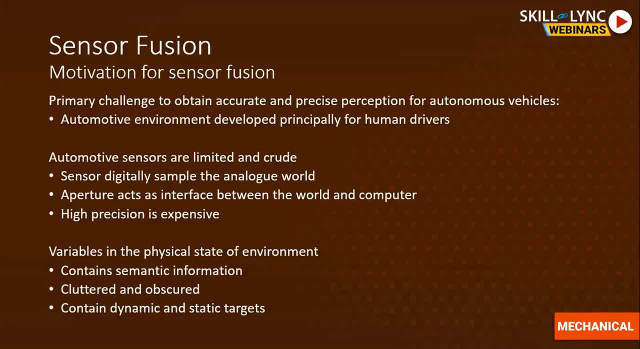 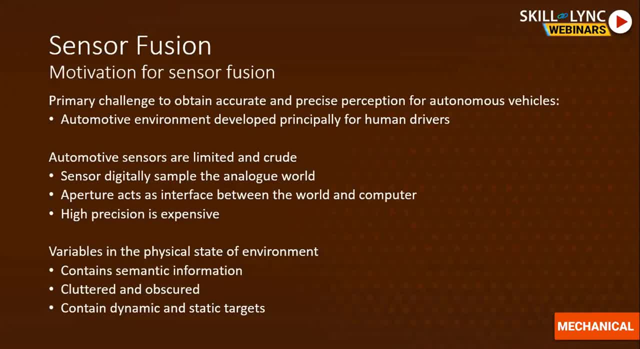 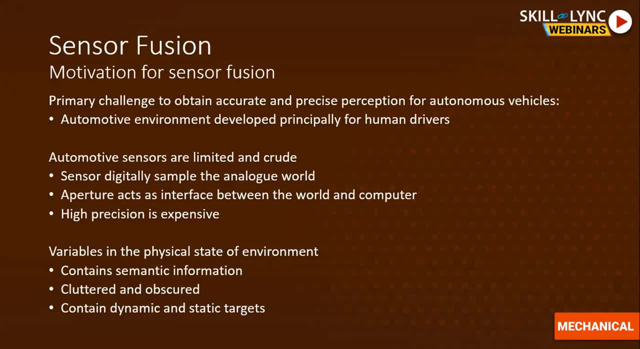 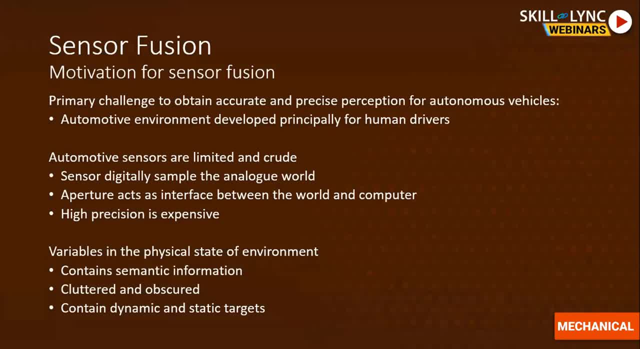 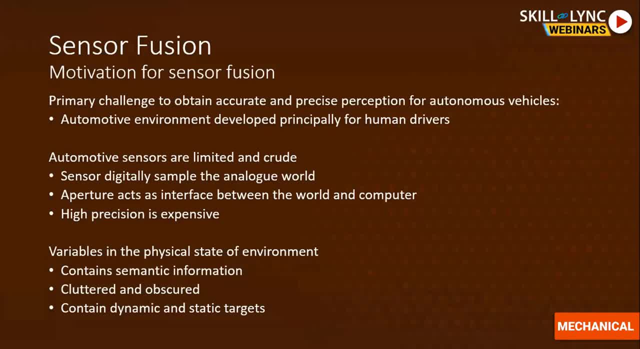 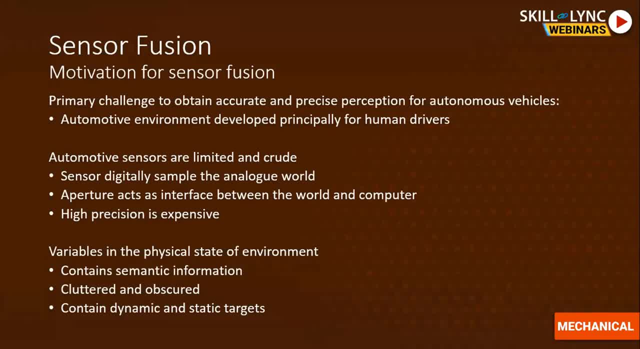 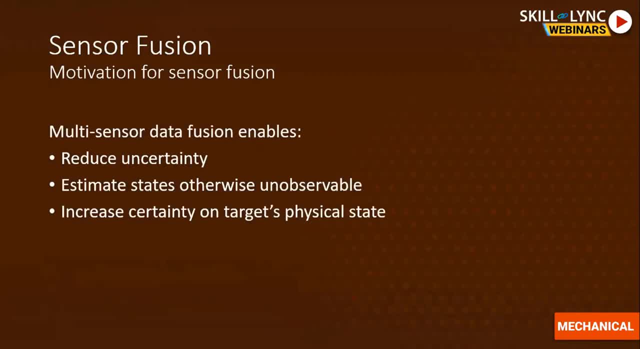 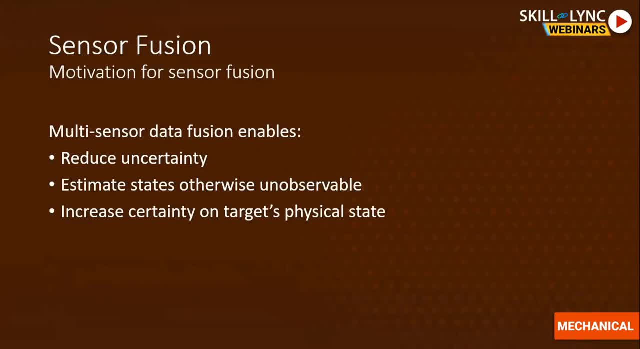 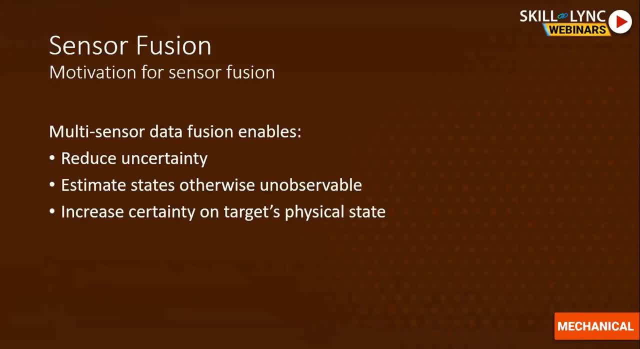 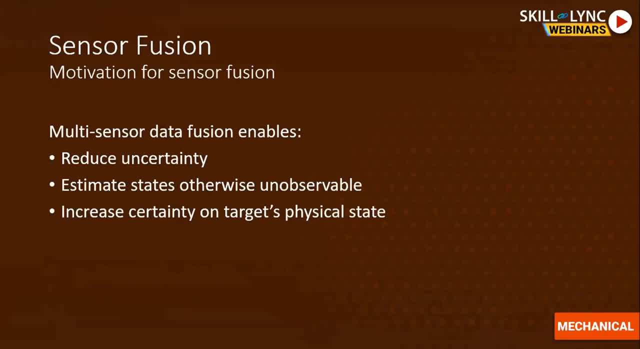 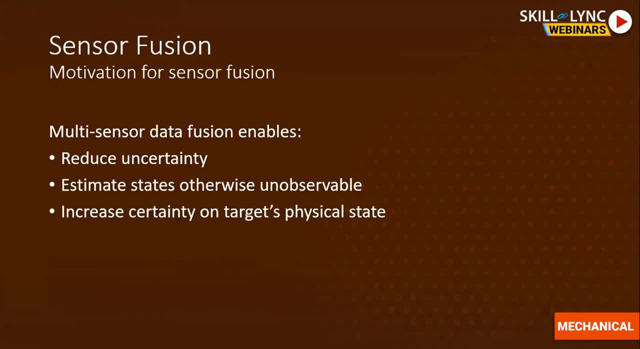 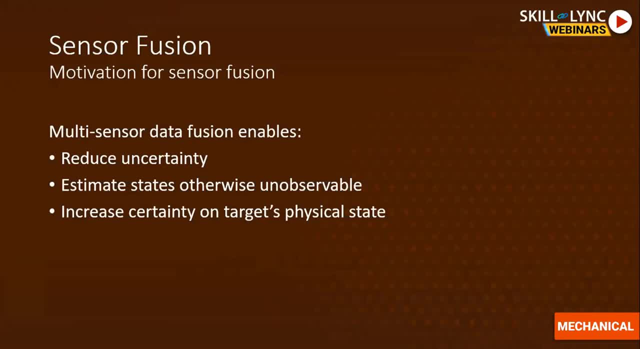 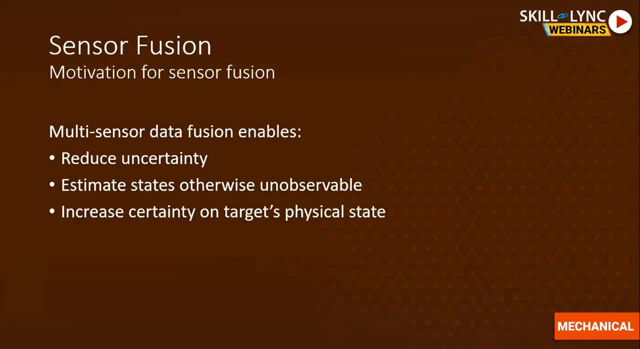 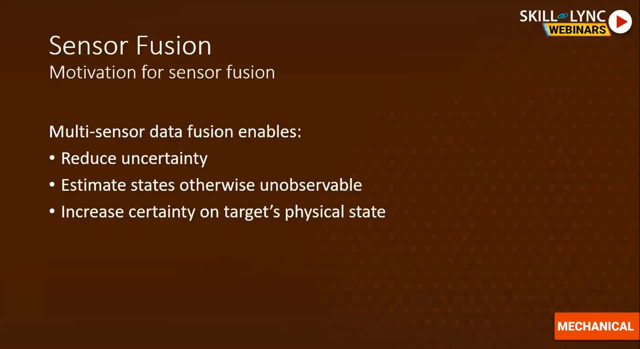 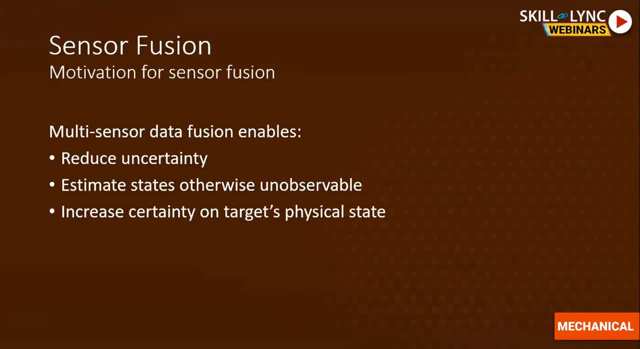 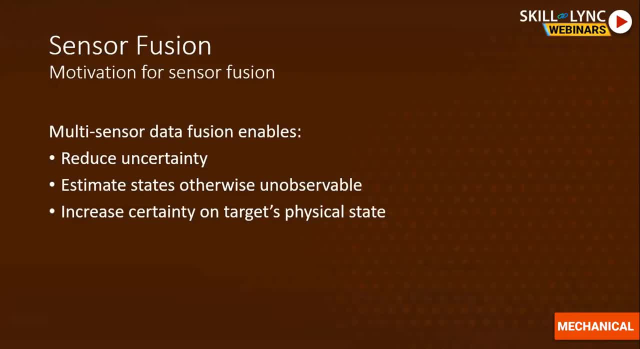 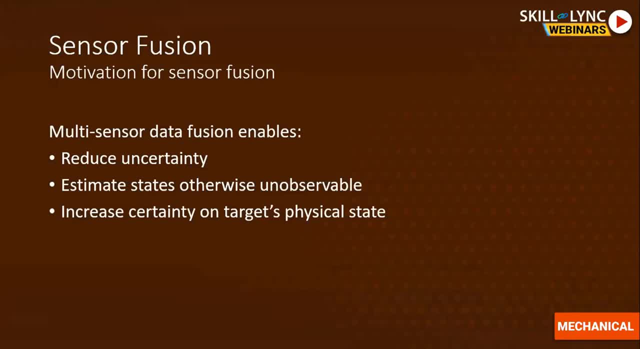 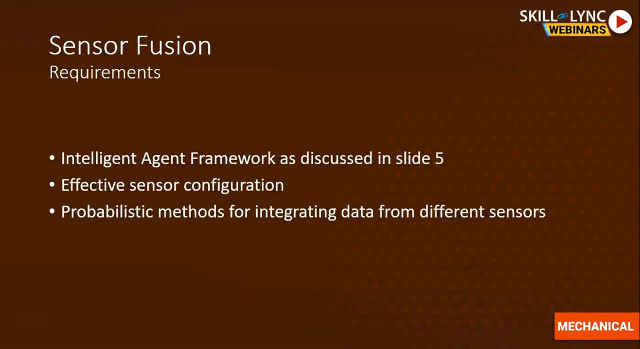 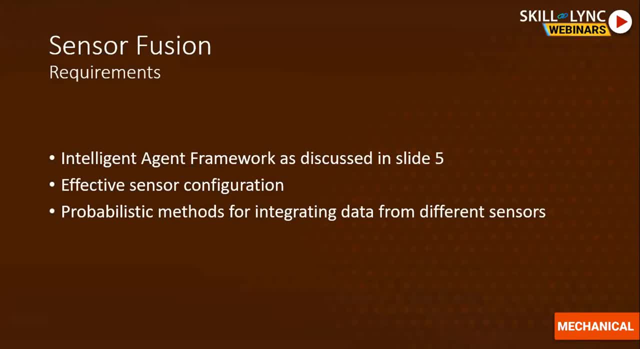 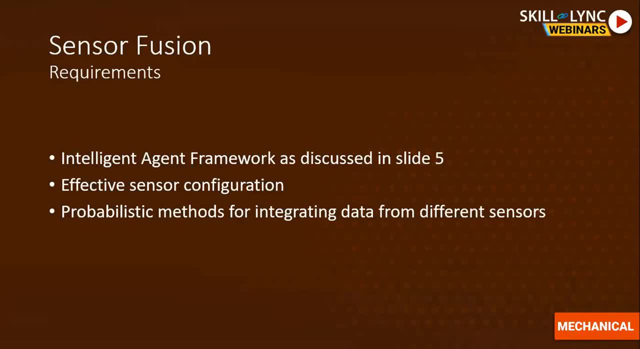 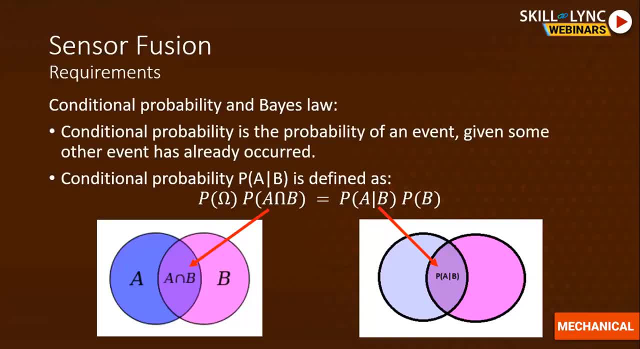 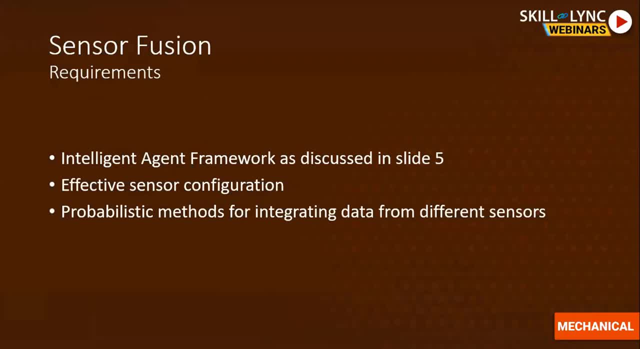 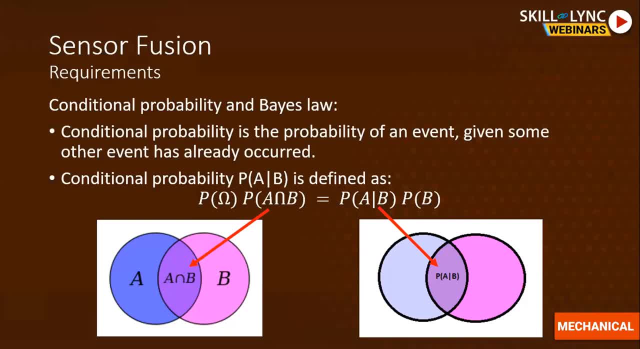 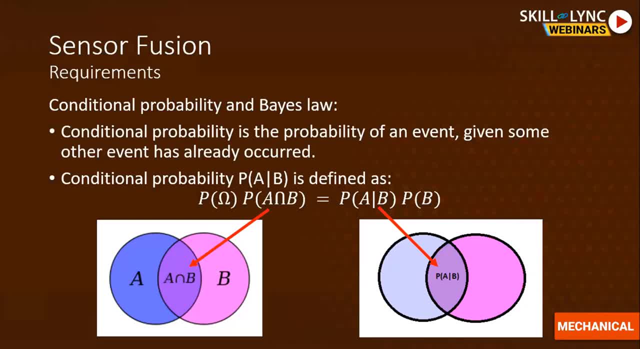 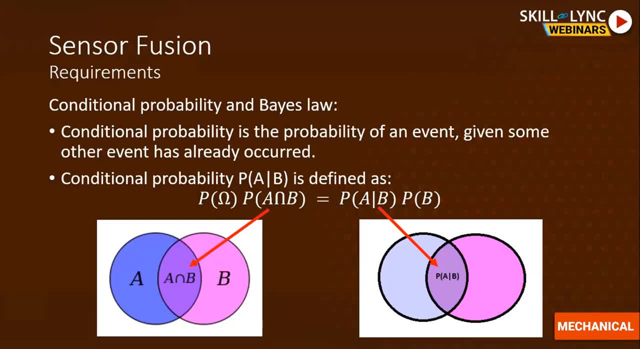 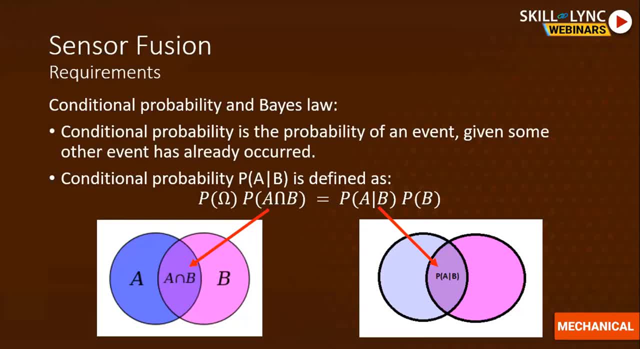 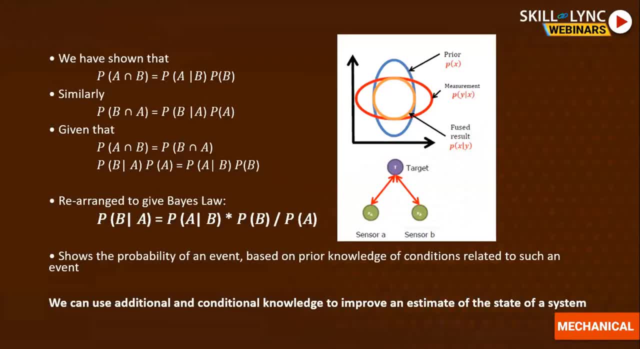 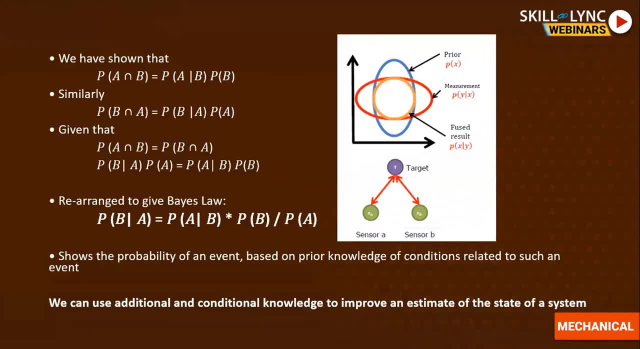 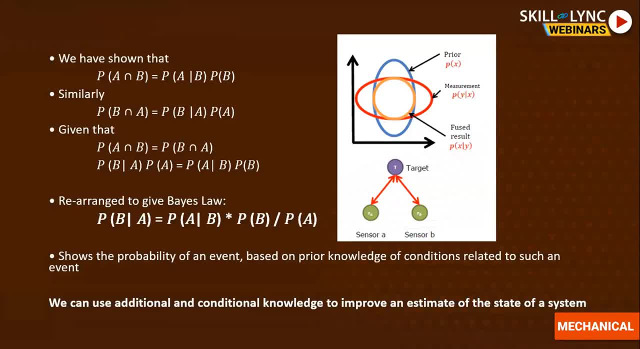 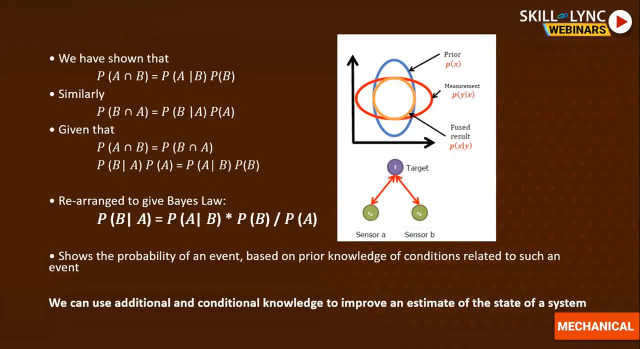